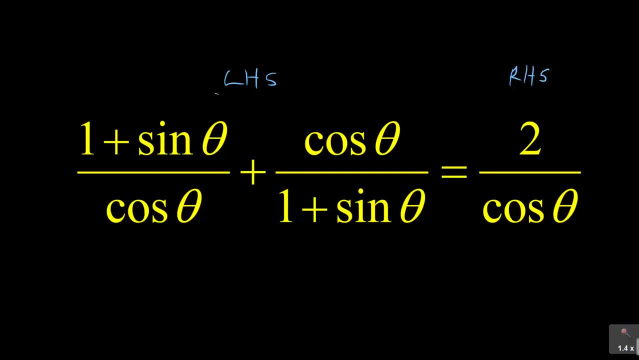 If you are going to start with the left hand side. If you are going to start with the left hand side, you must indicate I'm starting from the left hand side. Then your aim is to prove that the left hand side simplifies to become the right hand side. 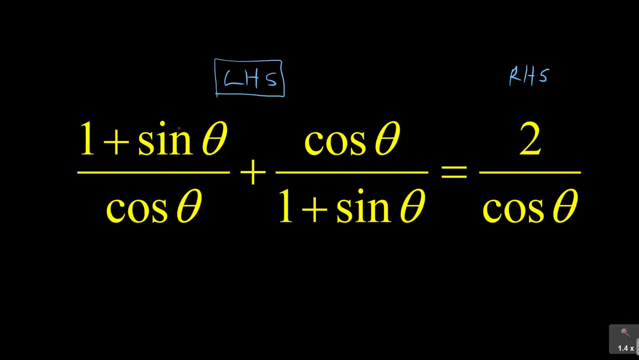 usually choose the side that is, that is more kind of. that is more kind of allowing you to work out. allowing you to work out or allowing you to do something else. you to simplify it further, For example, if I choose the right-hand side here, you can see that. 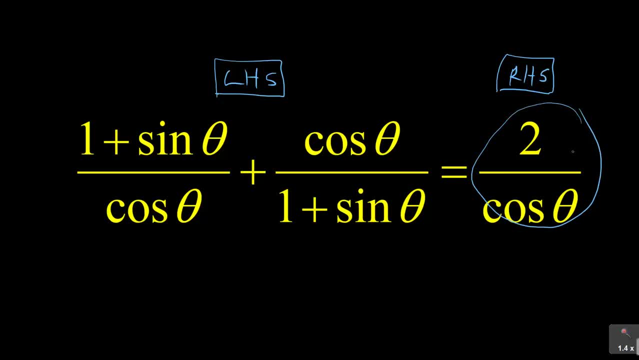 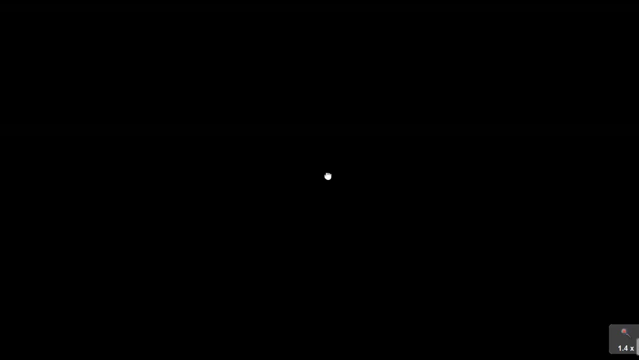 there is nothing much I can do here, So it is almost simplified. So it is good for me to choose my left-hand side in this case. It is not always the case that you choose the left-hand side, but you choose the side that works for you. So now, if I can just work it below, Now it is saying: 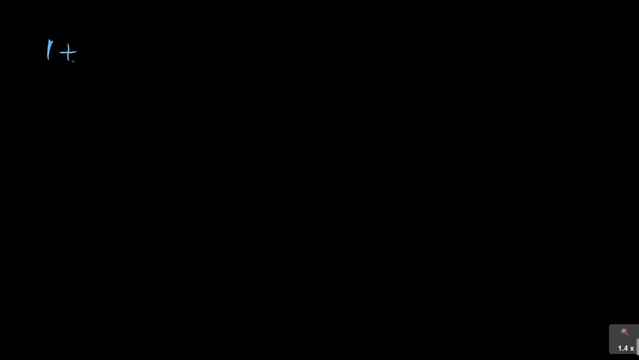 in this case 1 plus sin theta over cos theta plus cos theta over 1 plus sin theta. We must prove that is equal to 2 over cos theta. Let me just check. We are proving that is equal to 2 over cos theta. 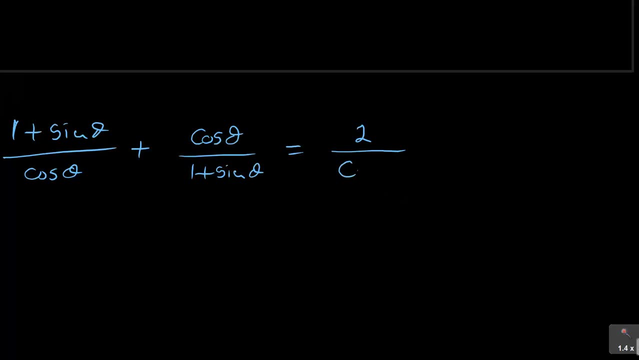 Not sin theta. So I've got this identity here, as you can see. So this is what I have And I need to prove, as I say, to choose which side you want to start with. So let me start with my left-hand. 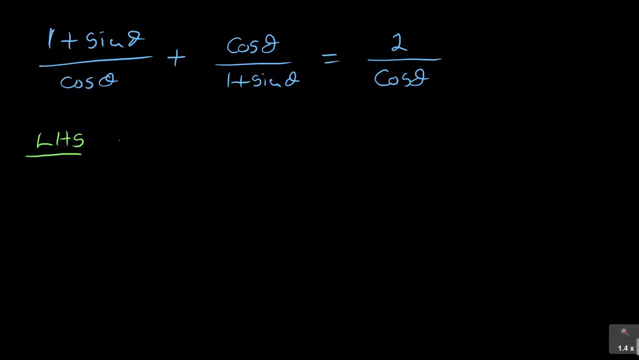 side And my left-hand side says 1 plus sin theta over cos theta plus cos theta over sin theta. Now, because I chose this side, I continue now working from that side. This is equal to. So, if I can use these two as my common denominator, I have cos theta And then I've got 1 plus sin. 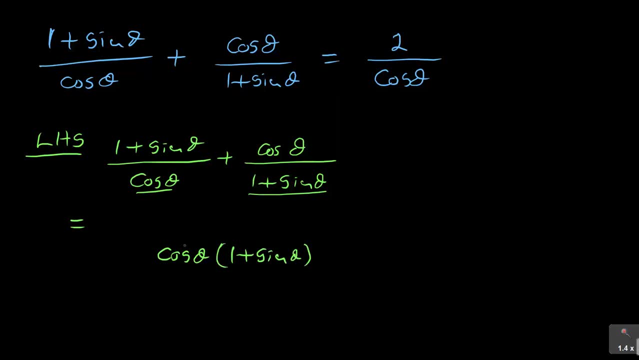 theta, But I need to protect that because it's got a positive sign as my common denominator. Now cos theta into cos theta plus 1 plus sin theta. So I've got 1 plus sin theta And then I've got 1 plus sin theta. Now students always confuse in terms of working with fractions. So what I'm doing 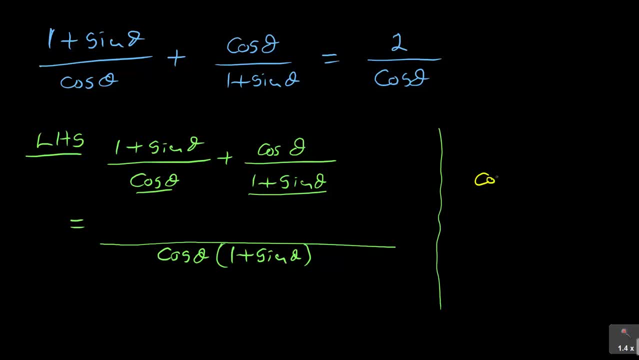 is- I'm saying this- my common denominator, which is cos theta, bracket 1 plus cos theta. This is my common denominator, So I'm going to divide it first by cos theta. So if I do that it will be over cos theta. Then when I cancel out, you can see 1 plus cos theta is remaining there, So I will. 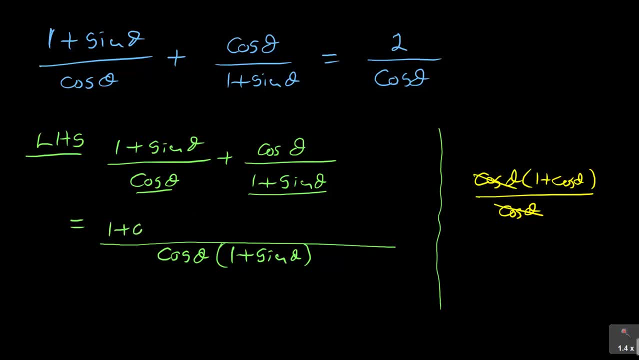 have at the top 1 plus cos theta. but it multiplies the top there and the top is in bracket 1 plus sin theta. So that is what is happening. You do the same thing here with the second one, the second one which? 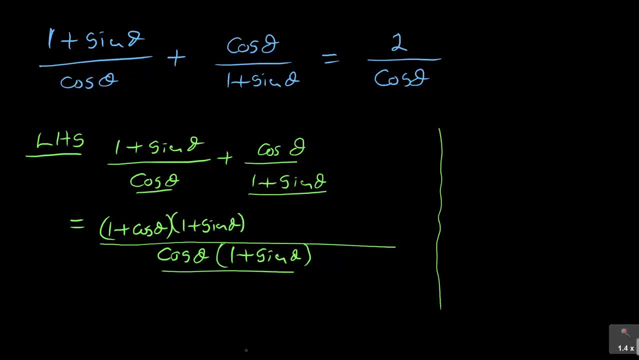 is 1 plus sin theta. So I'm using my common denominator again, which is cos theta. Just do a different mark, which is cos theta, 1 plus sin theta. But this time I'm dividing by 1 plus sin theta, which is 1 plus sin theta. You can. 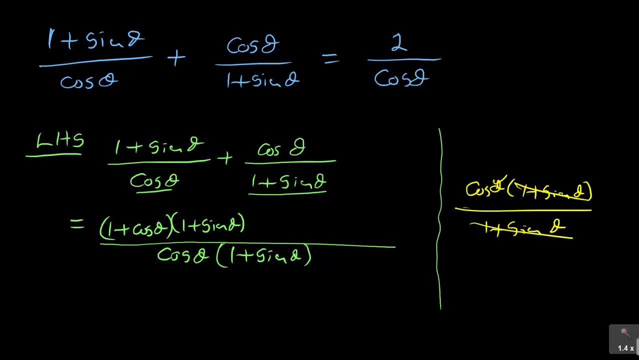 literally recognize it. when you cancel, you'll be left with cos theta. So you'll have that as cos theta, which is plus, because there's a plus sign, Cos theta, multiplying the top there and that particular top is cos theta. When you have done that, you can do the same thing here. So I'm 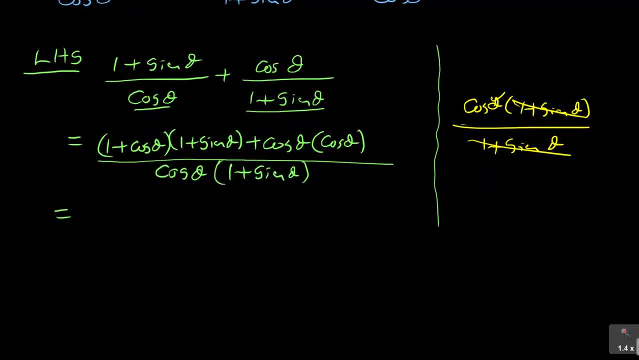 going to continue to simplify it, to say this is equal to open that bracket. In other words, you're expanding The first, one multiplies that, and 1 also multiplies that, Cos multiplies 1, and also cos multiplies sin. So it's a matter of expanding which is 1 times 1,, which is 1, plus 1 times sin, theta. 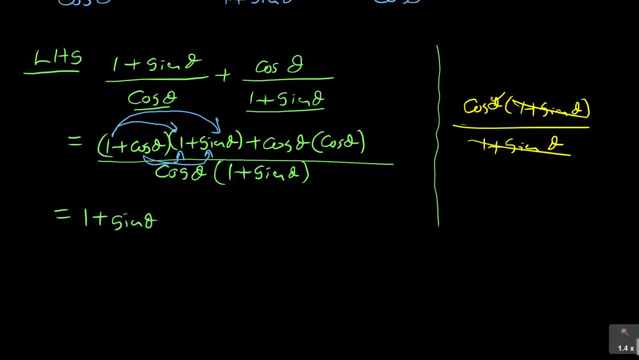 which is sin theta 1 times cos theta Plus cos theta and then cos theta. Actually, I yes cos theta times. I don't know where I got cos theta here. Let me just correct this, because there is no cos at all, but it is supposed to be. 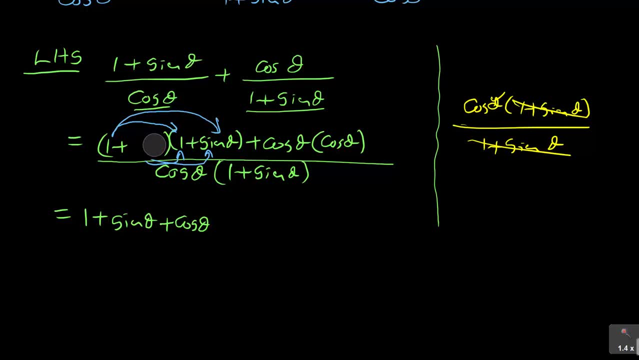 sin there. So please correct that as a mistake, because there was no cos at all. So instead it was sin theta there. So it's 1 times sin theta, which is sin theta, and then sin theta times 1, which is sin theta, and then sin theta times sin theta, which is sin squared theta. 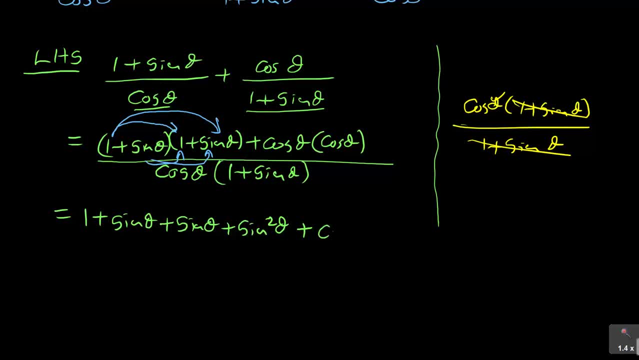 And then plus cos theta, times cos theta is cos squared theta for that part. Then I divide that by comma, So I get 1 denominator, which is cos theta 1 plus sin theta. Don't open the bracket at the bottom. Continue working on your problem Now. the next thing you needed to identify while you're working. 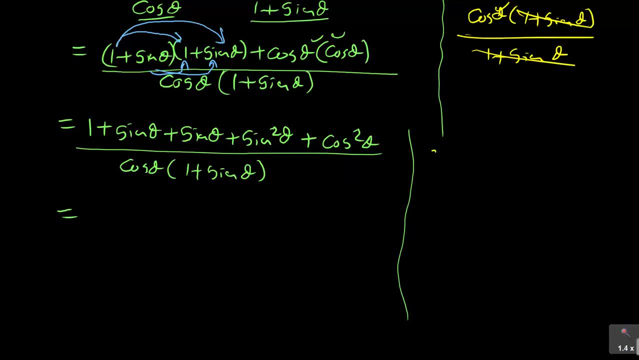 on this was this identity which says: sin squared theta plus cos squared theta is equal to 1.. Now check my videos where I prove this identity, because sometimes they can ask you in an exam to prove this identity. Now where is that part? Look at this part which says plus. You can see that. 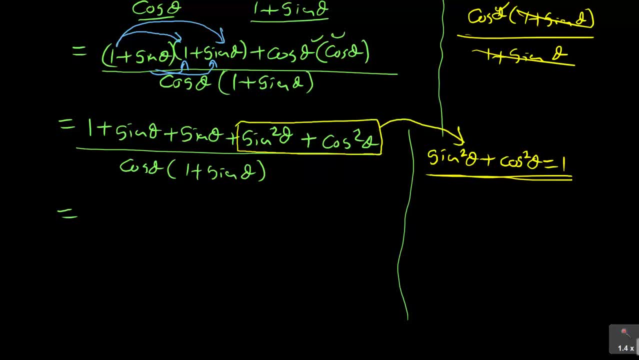 this identity is what I'm having here. So where there is that, you can substitute it with a 1 there, such that you've got 1 plus sin theta plus sin theta is actually there are two of them here, If you can check carefully. you've got this one and this one, So it becomes 2. 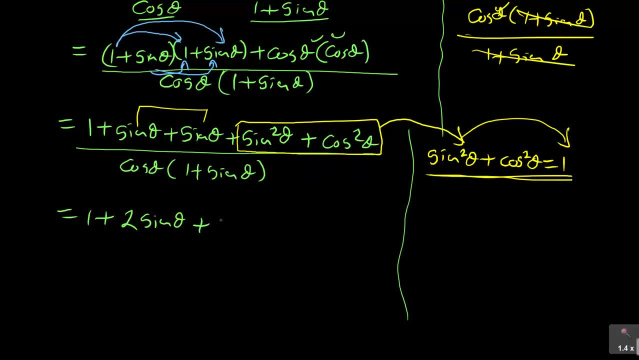 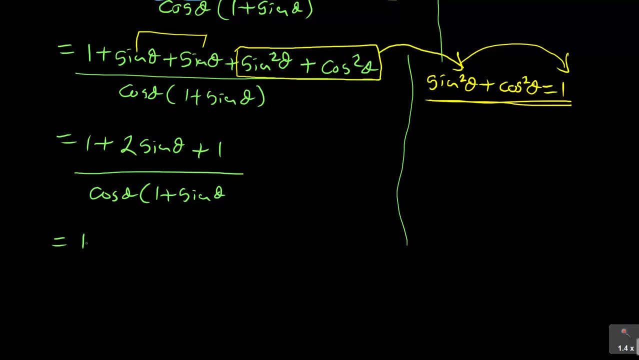 plus sin theta. plus. we said sin theta plus cos squared theta is 1 over cos theta. bracket 1 plus sin theta. Seeing that, and then you continue, this is equal to now you collect the like times, which is 1 plus 1.. 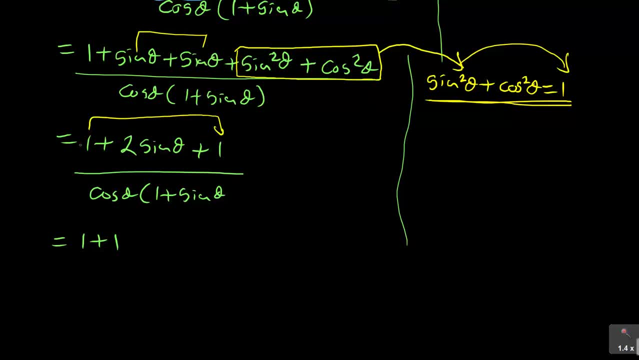 So what I'm taking is: I'm collecting that one and I'm collecting that one, So it's 1 plus 1 plus 2.. Sin theta plus sin theta, Sin theta plus sin theta over cos theta: 1 plus sine theta. 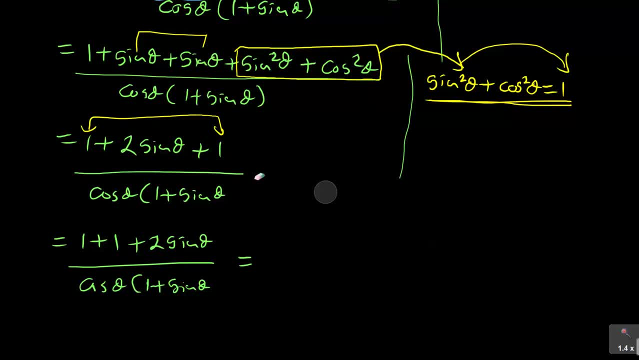 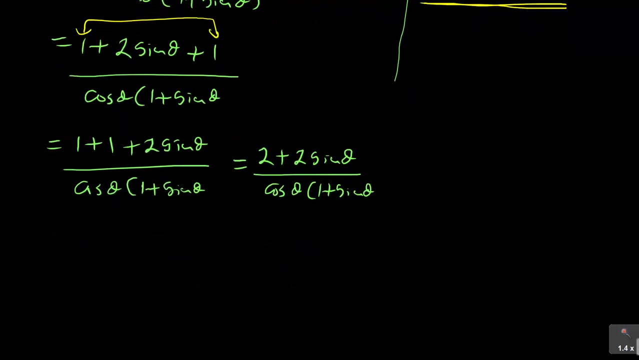 So if I continue now like that, it will be just wrapping it up. now, 1 plus 1 is 2 plus 2 sine theta, All right, Over cos theta into 1 plus sine theta, All right. And then when you conclude that: 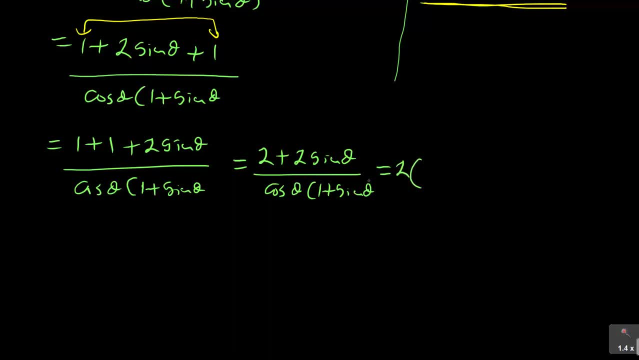 look at, 2 is common there I can factorize 2.. So when I take out 2,, 2 into 2 is 1 plus 2 into 2, sine theta is sine theta. Remember, when I multiply this 2 times, 1 is 2, which is that: 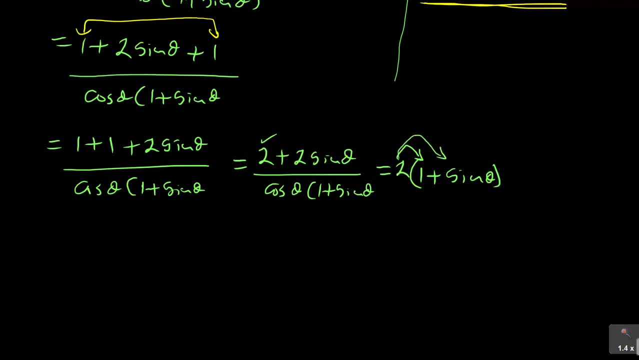 2 times 2 sine theta is 2 sine theta, like that. So that's why I'm saying: when you're factorizing, what you're simply doing is you're dividing 2 into 2, you get a 1., 2 into 2.. 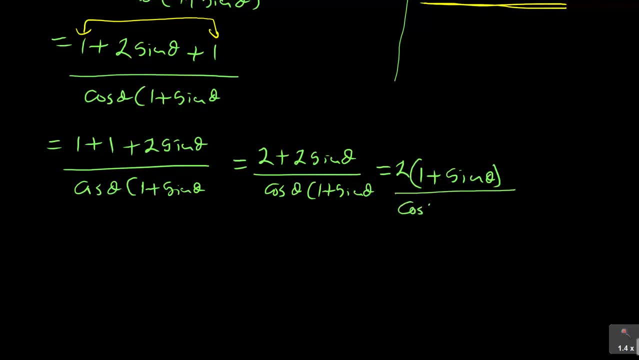 2 into 2 sine theta. is that All over cos theta, bracket 1 plus sine theta? I think you're already seeing what this is going to. This cancels, this cancels, And what we are left is equal to 2 over cos theta. 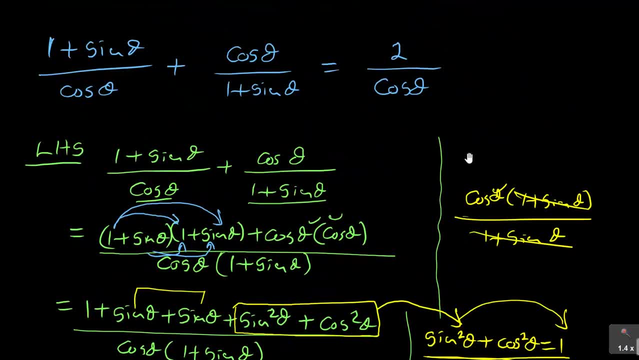 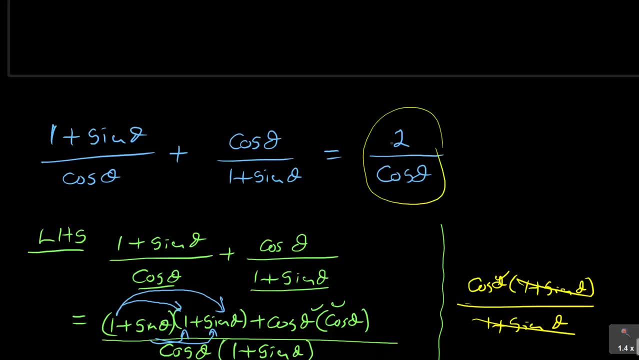 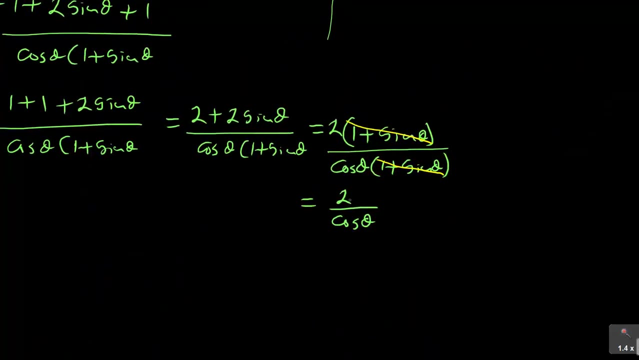 And if we go to the original, they say we must prove that this is equal to 2 over cos theta. from our, from our question, And if I can just further confirm, yes, 2 over cos theta. So you can see that this has proven that it is equal to 2 over cos theta. 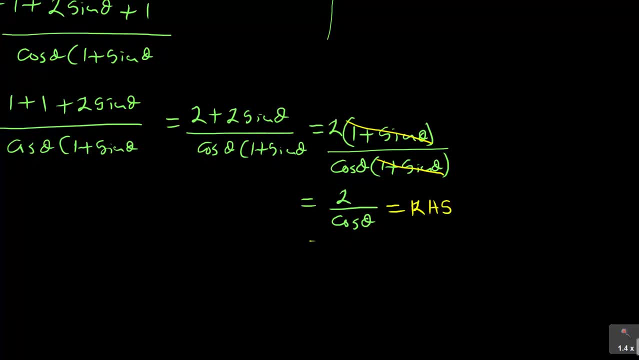 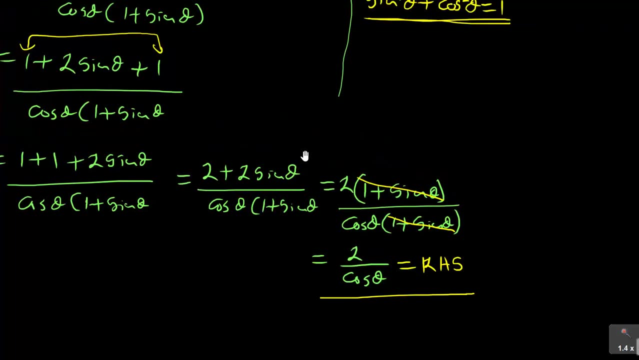 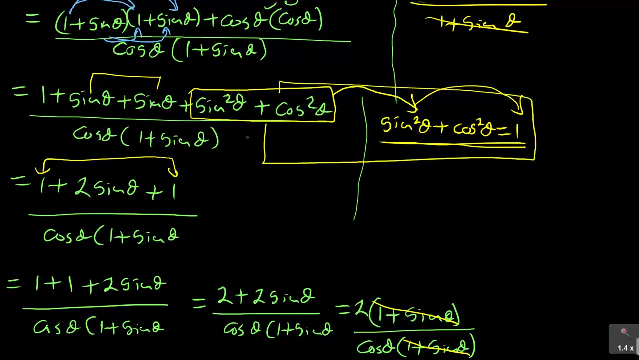 which is equal to right hand side. So we have managed to prove that identity. So this is how you can use some of this part, because the most important part was you recognizing this identity. It was going to actually frustrate you if you didn't know that identity, as well as being able to factorize. 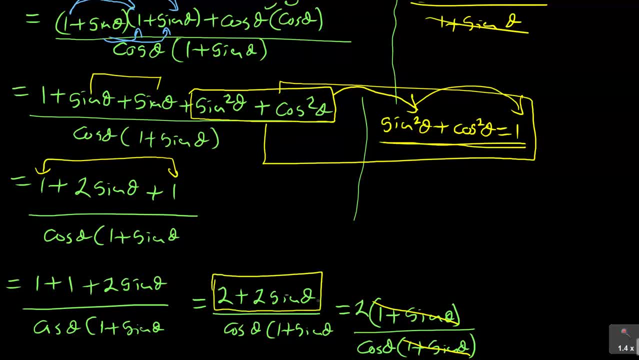 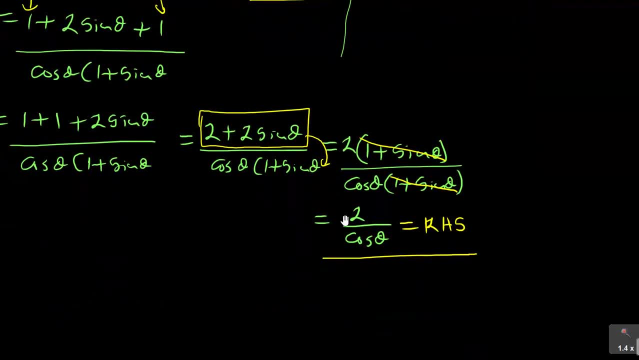 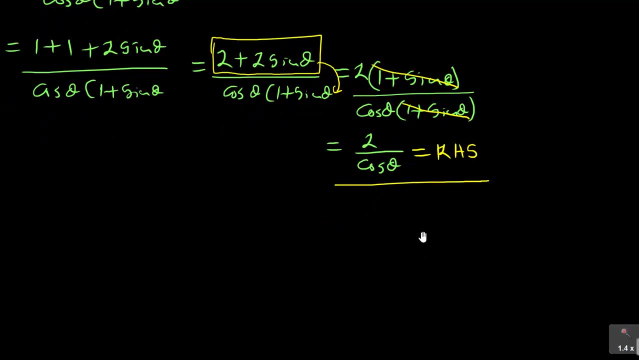 Here was the highlight to identify that this cancels with that one at the bottom there. So these are things that are strategies that you can use whenever you're doing your proofs And, as you continue, I'll check our lessons. I'll bring more and more of these proofs time and again. 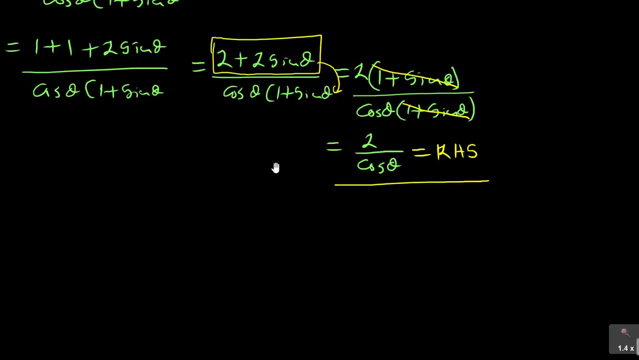 That's why I say you need to subscribe to our channel or like our page. whenever there is a new video that we've posted, you'll be notified and check whether it also talks about these kind of problems, And this will actually assist you as you prepare for your final exams. 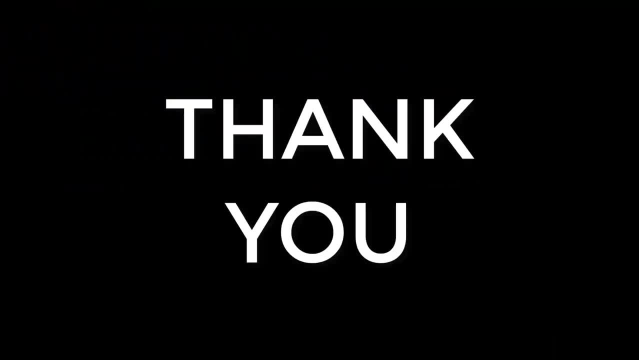 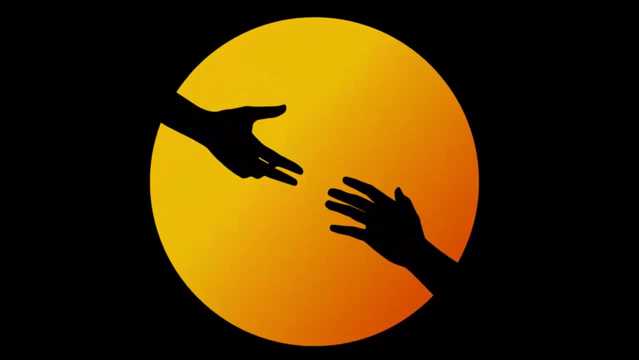 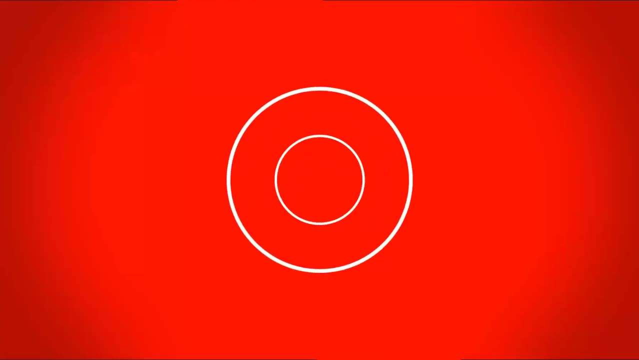 We have come to the end of our lesson. Thank you. See you next time.